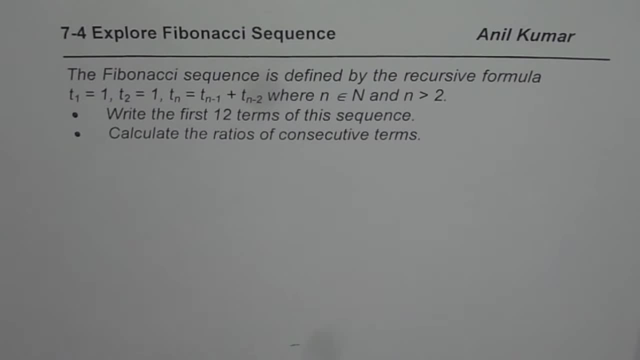 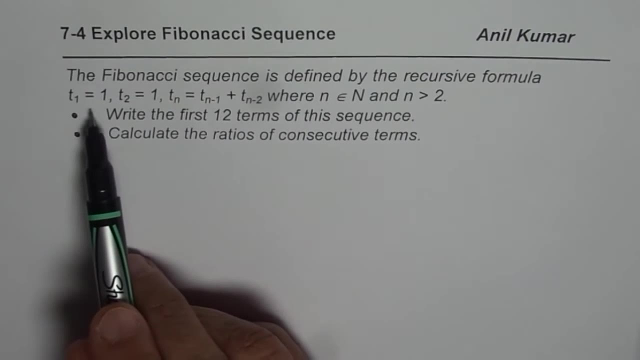 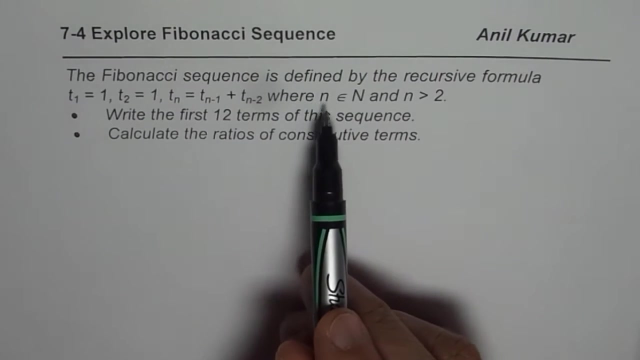 So let us explore Fibonacci sequence now. The question here is: the Fibonacci sequence is defined by the recursive formula: t1 equals to 1, t2 equals to 1, tn equals to tn minus 1 plus tn minus 2, where n belongs to set of natural numbers and n is greater than 2.. 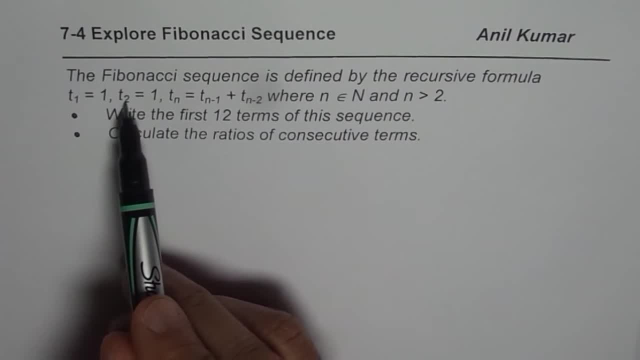 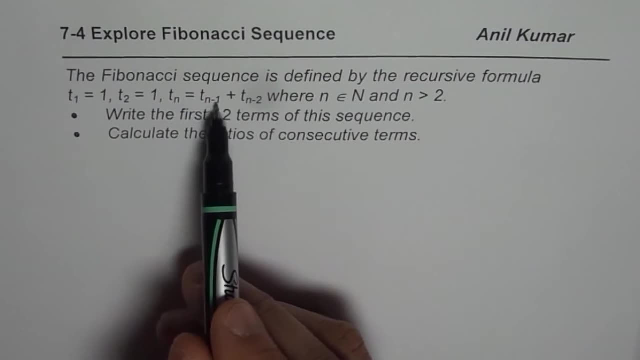 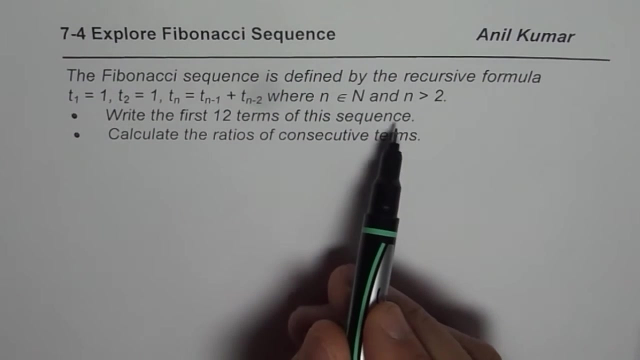 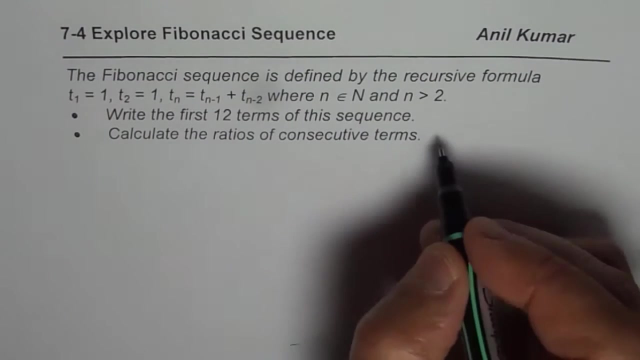 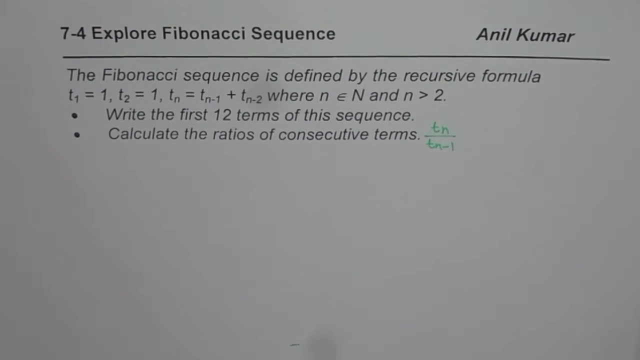 Now it makes sense: n equals to 1, n equals to 2 is already given to us as 1 and 1.. So the next term can be found by a combination of previous two terms. So that is the sequence. Now we need to write the first 12 terms of this sequence. That's the first part, And second part is calculate the ratios of consecutive terms. That means we have to find tn over tn minus 1.. Correct, So that is what we need to figure out, And what we will see is that this ratio approaches the golden ratio. 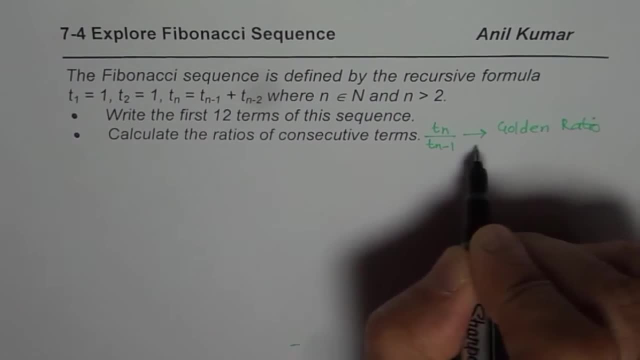 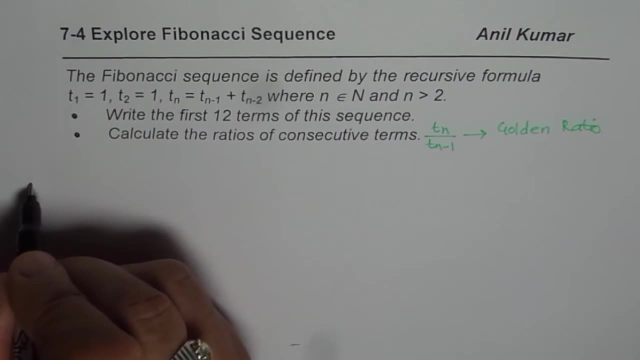 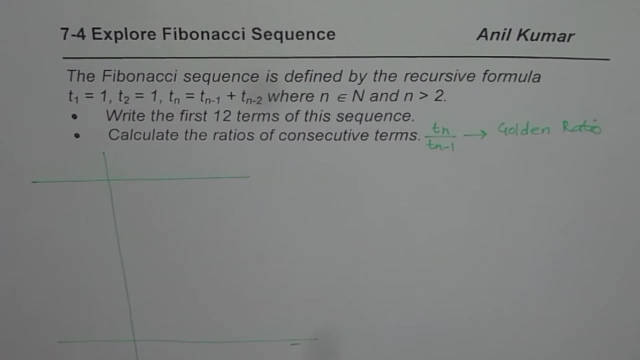 that is how my videos are connected. Okay, so keep that in mind that this ratio actually approaches golden ratio. We'll also find what is golden ratio, Okay, so let's begin by finding the terms first. Okay, we have very limited space. that is the boundary. Okay, let's write down all the terms. 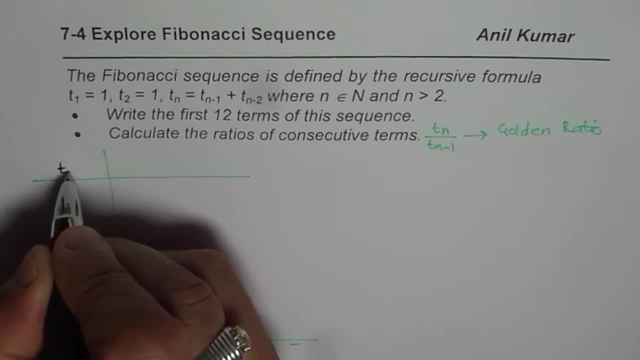 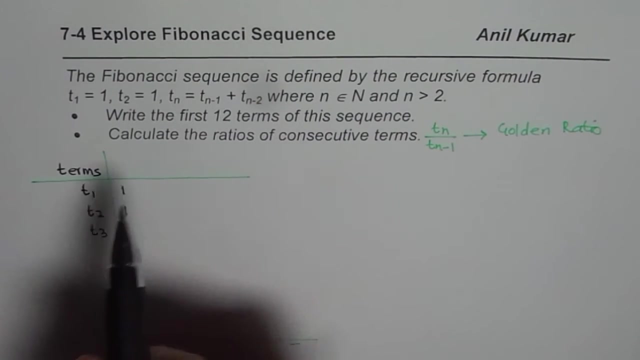 first. So we are saying terms right. So let us say terms here. starting with the first term: t1 is equal to 1. for us, t2 is also equal to 1.. The series is generated by adding previous two terms. that is the meaning of tn minus 1, previous term, n minus 2, previous to previous, correct. 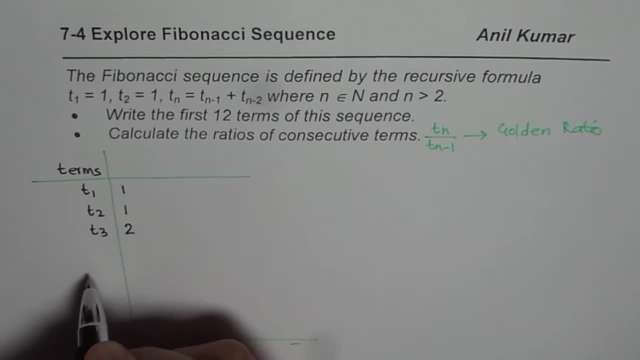 So previous two terms. add them up to get the next term. we get 1 plus 1 as 2.. So it is very easy to generate this list of sequence: See t4,. just add 2 and 1, you get 3, t5, 3 plus 2, 5, t6, 5 plus 3, 8, t7, 8 plus 7, 13,. right. 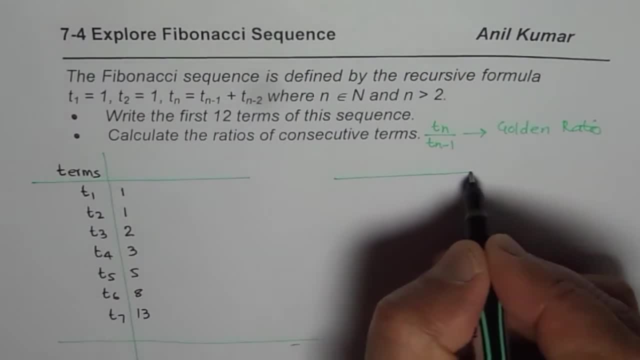 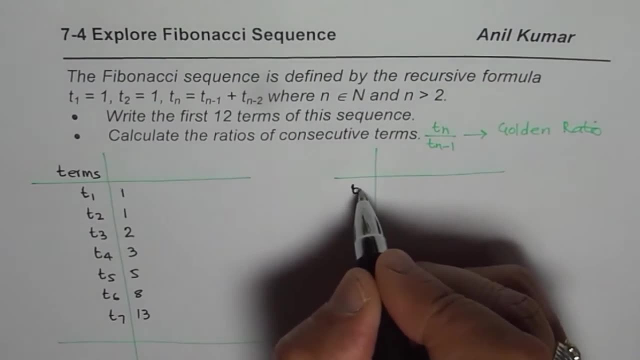 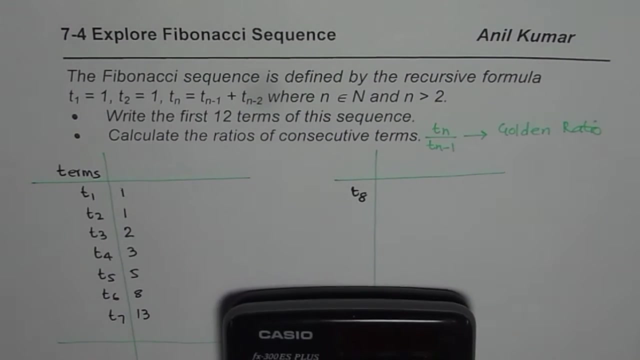 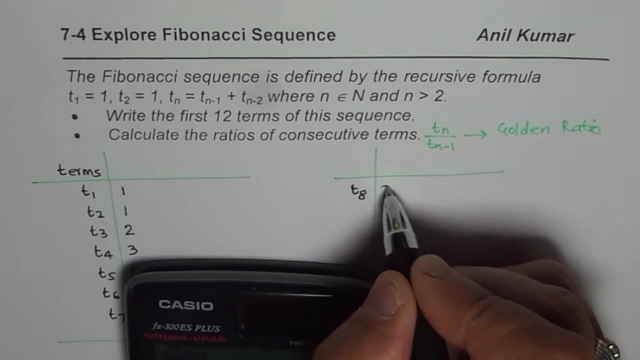 So let me add more terms and I will do the late, this half of the page. Okay, so we'll write t8, t8 will be t6 plus t7.. Let me use calculator, because if something goes wrong then everything will be wrong. So 8 plus 13,- previous two terms we have to add, we get 21.. Now to 21,. 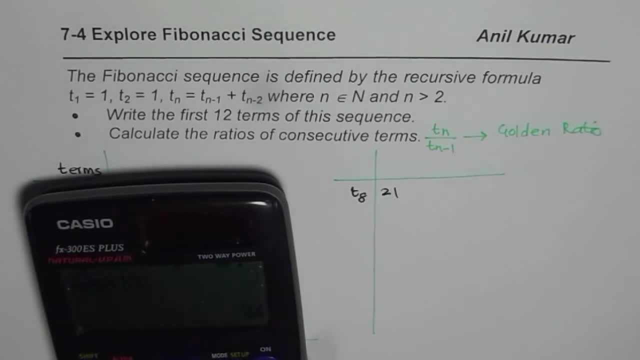 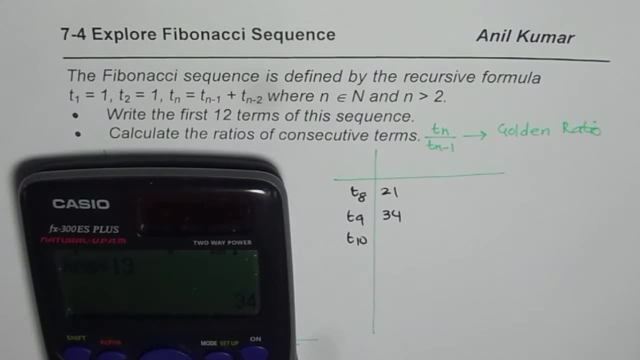 we add the previous term, which is 13,. right, So 13 equals to 34.. So we get t9 as 34.. t10 will be 34 plus 21,, right, 55.. t11 will be 55 plus 34,, that is 89.. 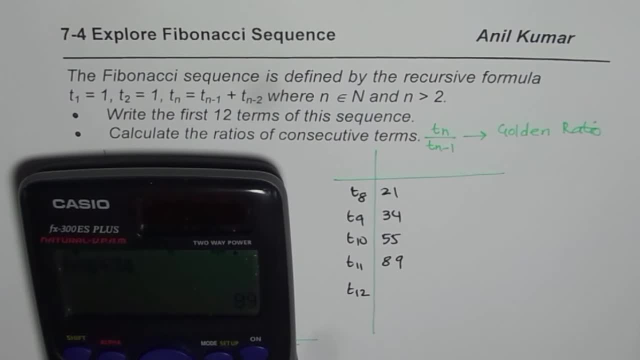 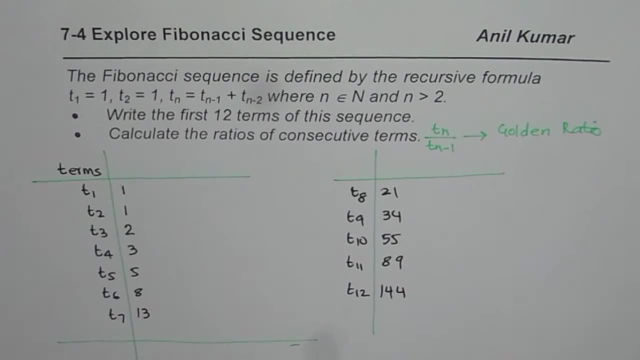 See how easy it is. t12 will be: add 55 to 89,, 144.. That's a good number to stop. Okay, 12 squared is 144, so I think we are at the right place. 12 squared is the 12th term. 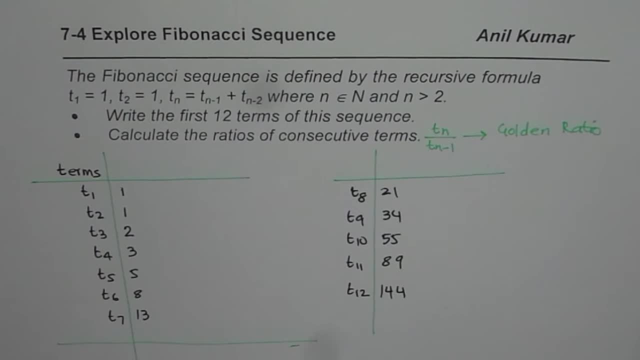 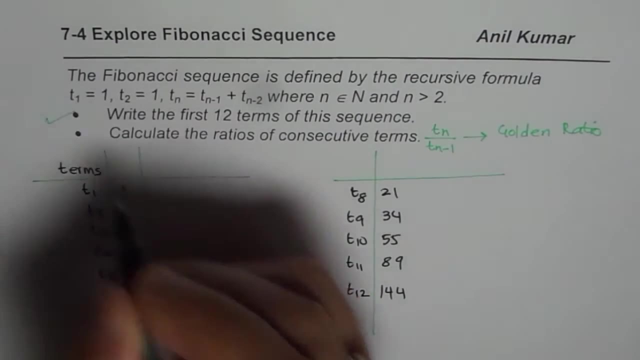 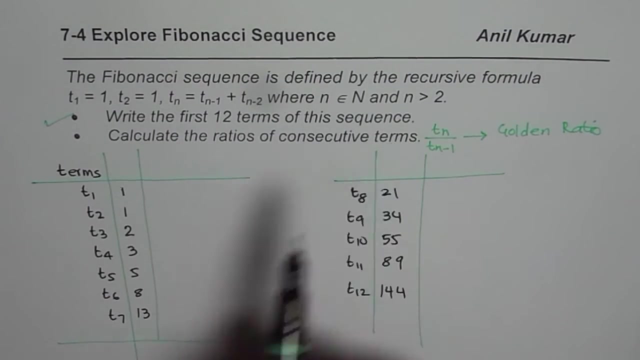 So that is another way to check whether we are right or not. Okay, now we have to find what is the ratio. So we have done the first part right. So we already have the 12 times 12. 12 terms in a sequence. Calculate the ratios of consecutive terms. That means we will do. 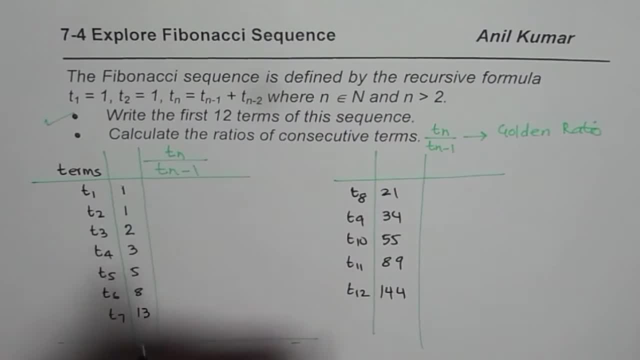 tn divided by tn minus 1.. So let me write down what I mean. It means 1 divided by 1.. This 1 divided by the previous one, So 1 over 1, which is equal to 1.. Then we write 2 over. 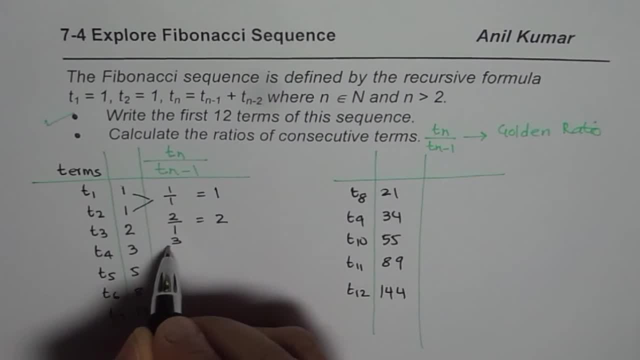 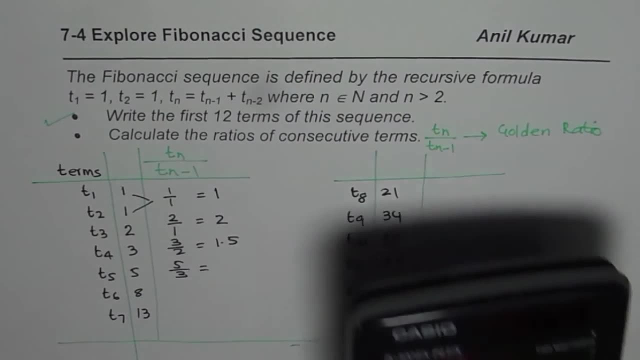 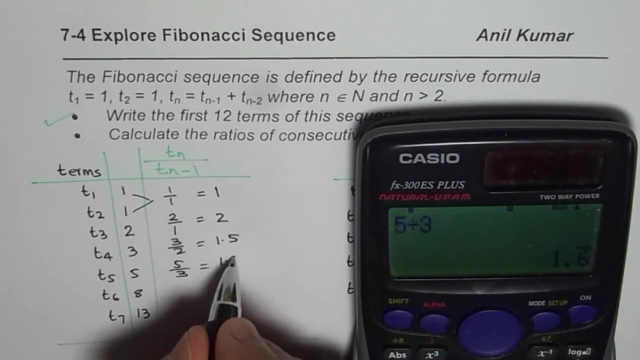 1, which is equal to 2.. 3 over 2 is equal to 1.5.. Then 5 over 3 is equal to – let's take help of calculator. So we have 5 divided by 3 equals to, in decimals, 1.66.. Now we'll do 8 divided by 5.. So we have 8 divided by. 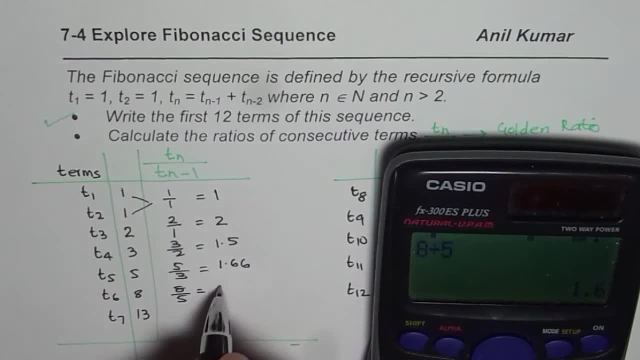 5 equals to, in decimals, 1.6.. You'll find now: the first decimal place is constant, 1 is the whole number which is constant, correct? So we have now 11 plus 12.. Because the first decimal place is constant, 1 is the whole number, which is constant, correct? So we have. 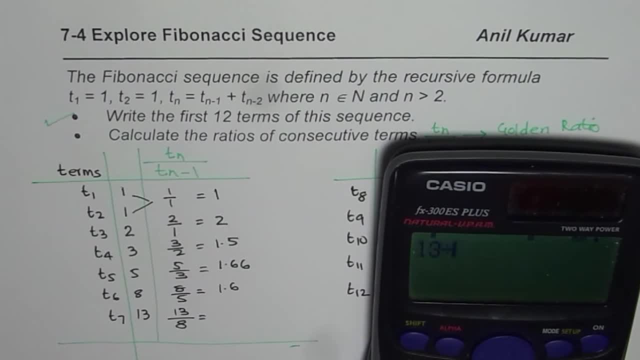 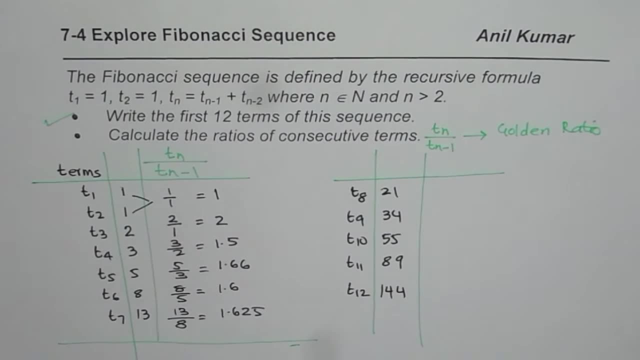 now 13 divided by 8.. 13 divided by 8 equals to, in decimals, 1.625.. Now you observed that first decimal place is 6, right? So we have 1.6 as a constant for each ratio as we move. 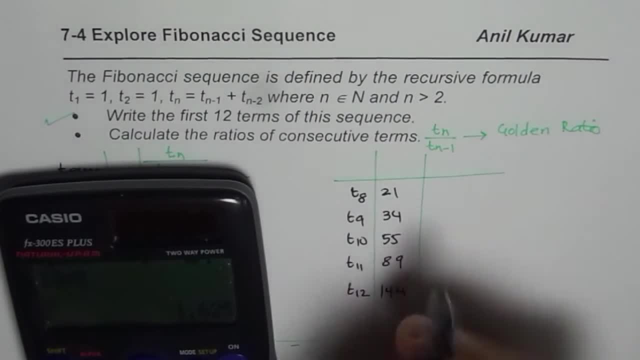 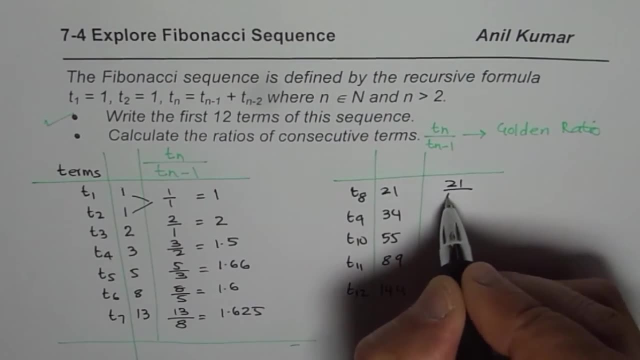 forward. Let's do this part, which is: did we take care of 21?? No, 21 divided by 13,. right, So we'll do 21 divided by previous number, 13.. So 21 divided by 13 is equal to. 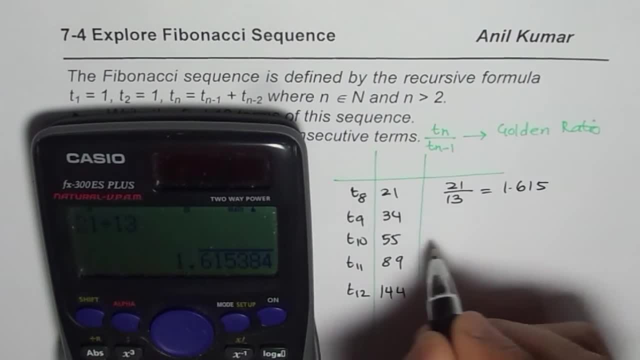 in decimals: 1.615.. So now we have 34 divided by 21.. It is an interesting exercise, just take some time: 1.619.. 55 divided by 34 equals to divided by 34. equals to divided by 34. 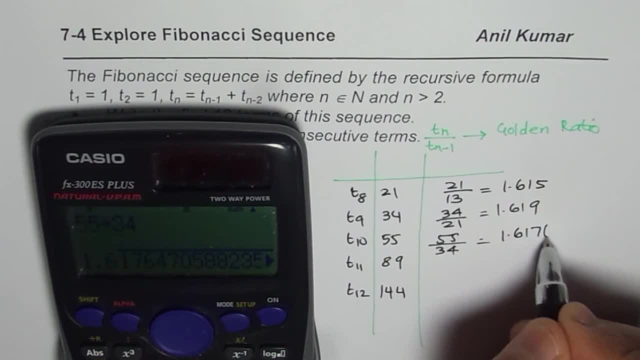 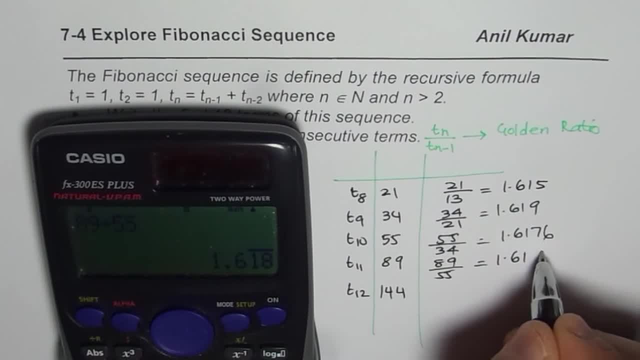 to in decimals 1.618.. Now you see, 61, 6161 is constant. And now let's do 144 divided by 89.. 144 divided by 89 equals to in decimals 1.6176.. And then we have 84 divided by 89. 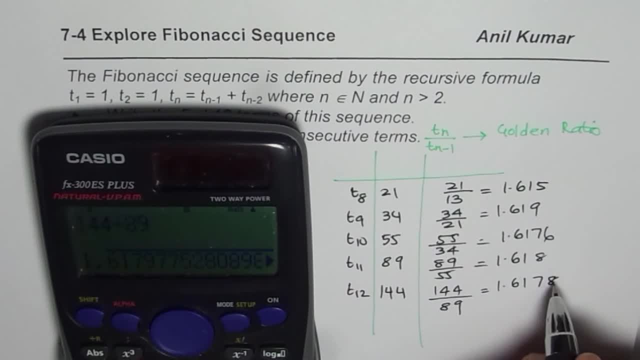 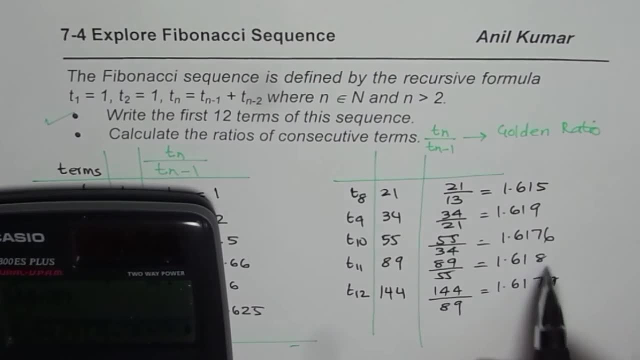 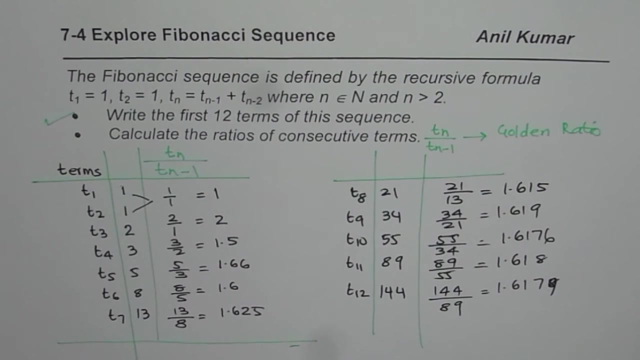 equal to 1.6179.. It is. it is approaching 8.. Do you understand 1.618,? it is approaching 79. Do you get the idea? So what we find here is that the ratio approaches 1.618 as we move. 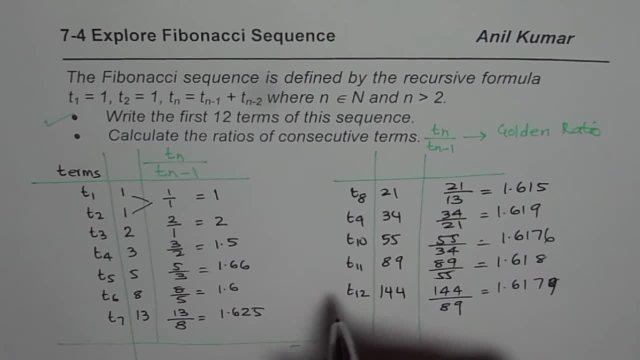 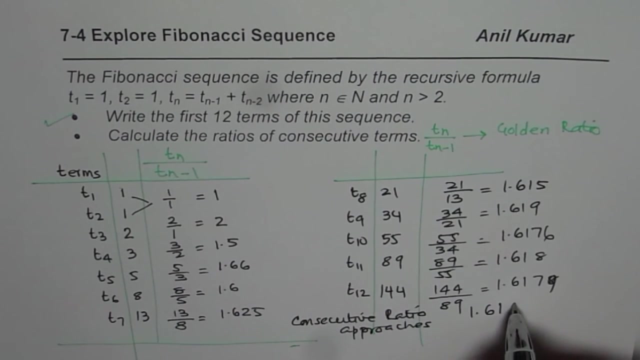 forward right. So we see that the consecutive ratio approaches 1.618, so that is what we see from the ratios of first 12 terms. If you continue this sequence, you will get one particular ratio, and this ratio is the golden ratio which we are talking about.